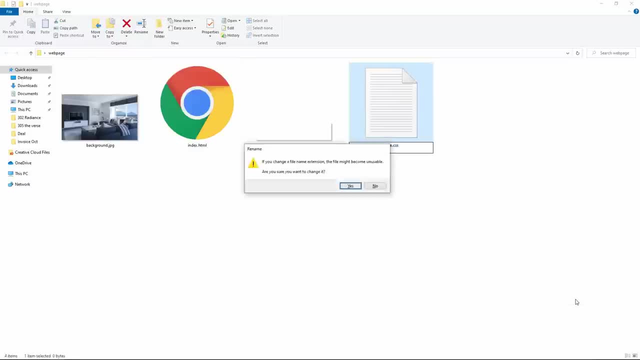 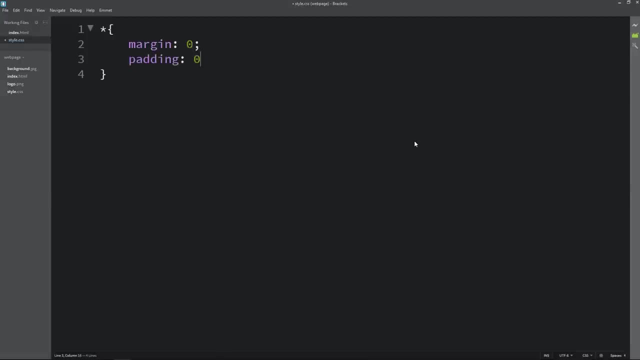 to the folder again and create a file and rename it as style dot CSS. open this file with text editor and here we will add star margin 0 and padding 0 and font family. next we have to connect the HTML file with the CSS file. so we will come. 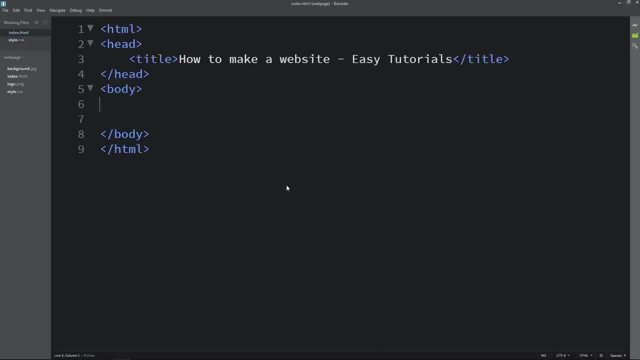 back in the HTML file, and here in the head tag we will add link rel. styleset href is equal to file name of the CSS file, which is style dot CSS. next we will write the code in the body tag and here we will create one tip with the class. 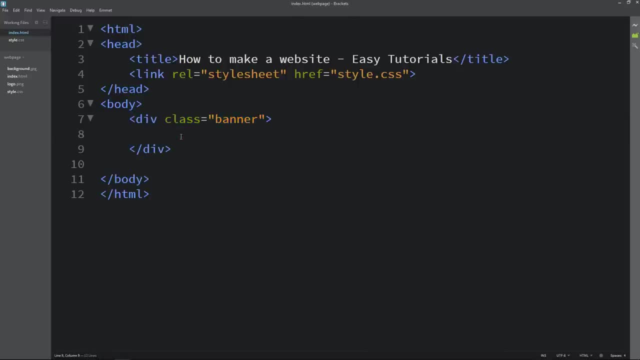 name banner. next we will create a class name banner and here we will create a copy. this class name banner and come to the CSS file. add it here with the dot. here we will add the width and height. next we will add the background image. here I'm adding linear gradient and this color code, so it will add a colored. 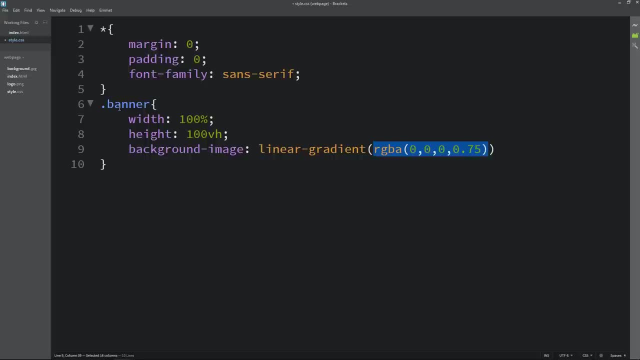 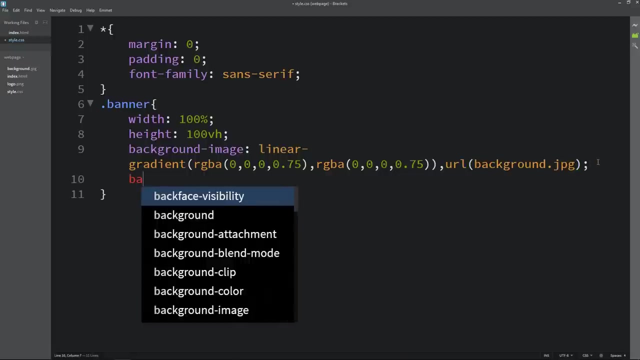 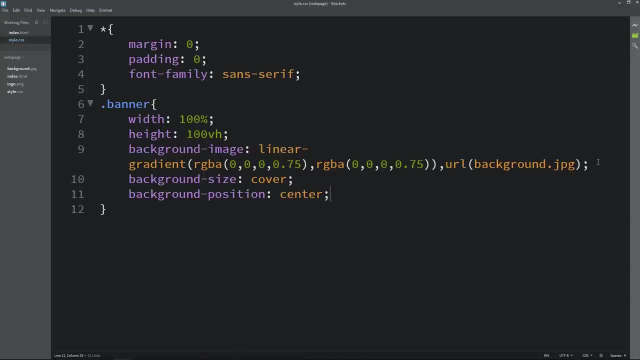 layer over the image, then write URL and the image file name. so the image file name is background dot jpg. after that we will write background size, it will be cover and background position will be Center. after adding this again, come back to the folder and open this HTML file with Google Chrome and you can see one. 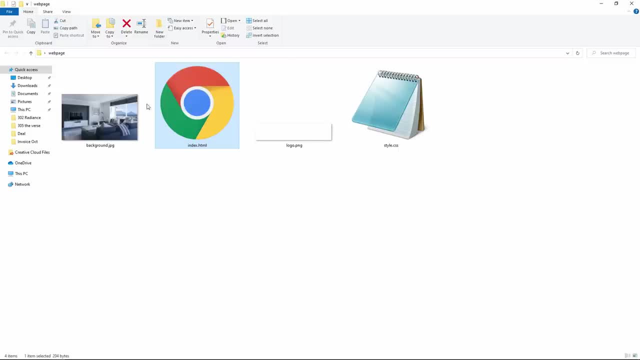 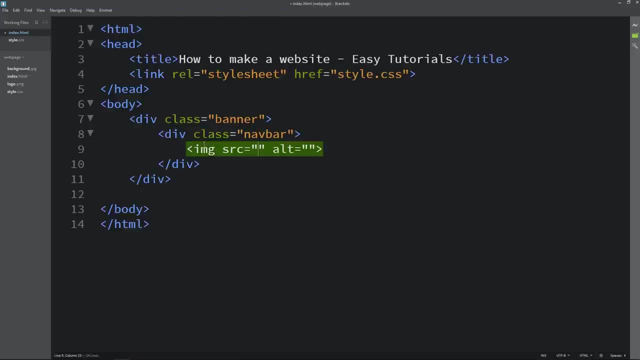 image on complete web page. next we will come back in the HTML file and here we will create another div with the class name navbar. in this div we will create one logo- so I am using img tag and the file name is logo- and one class name which is logo. after that we will add some menu. so here i 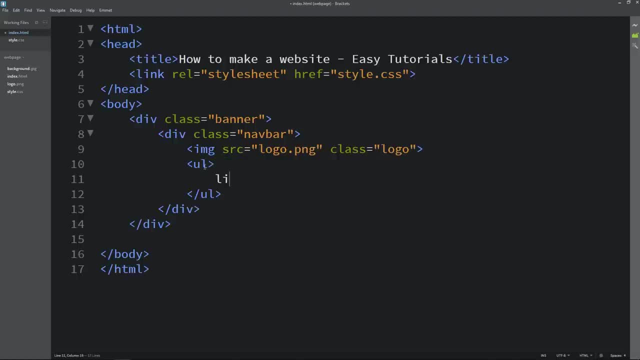 am adding ul and li, then anchor tag and the anchor text will be home. simply duplicate this line and change the link text. it will be bedroom, dining, kitchen and backyard. so we have five links. you can see the logo and links on the web page. next we have to add: 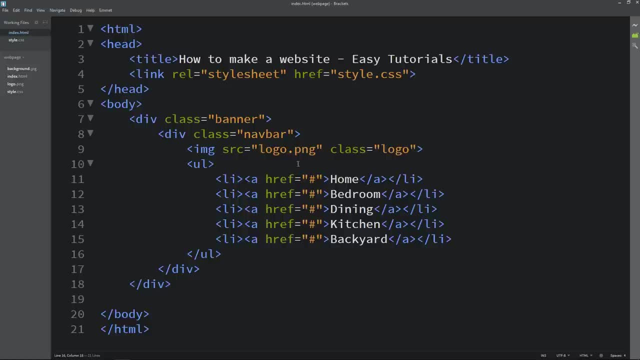 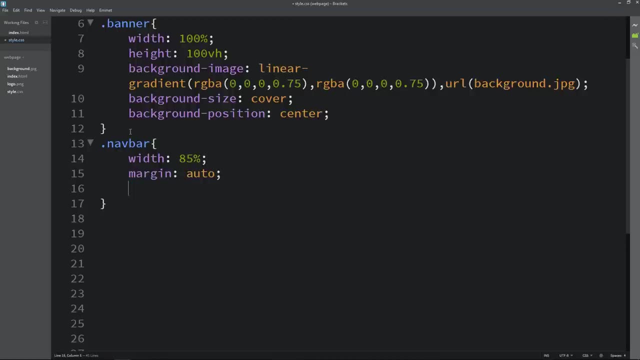 some space from the left and right side, so just come back and copy the class name nav var. write it here in the css file. for this one we will add the width 85 percent and margin auto and padding 35 pixel and 0. display will be flex and align. item center. justify content. 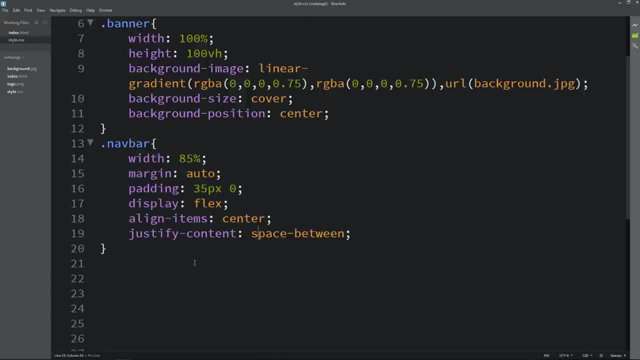 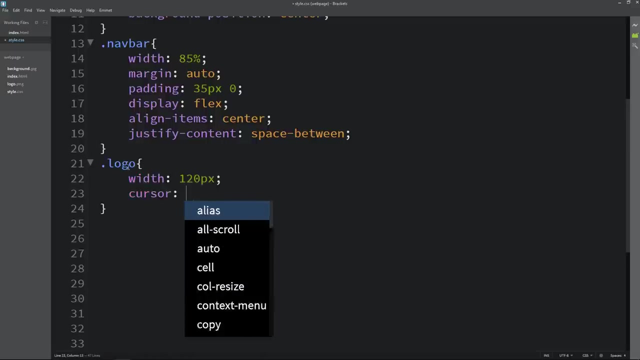 will be space between now. you can see some space from the left and right side, and the menu is in the right side. now just come back and copy this class name logo. write it here for this one. we will set the width and we will add cursor pointer. now we will write. 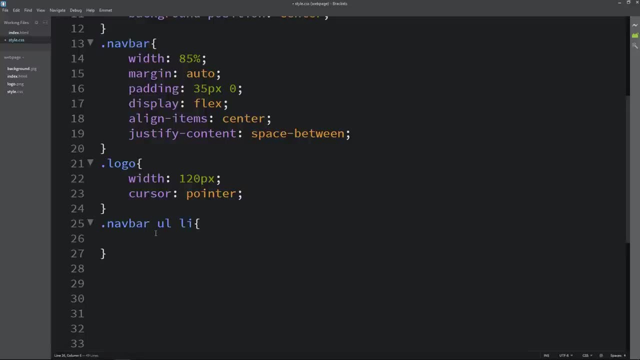 the code for the menu. so copy this one, then write ul and li for this list. we will add lister style: none, display, inline block and margin. you can see some space between these menu. next we have to change the color, so just come back and copy again. then write a for. 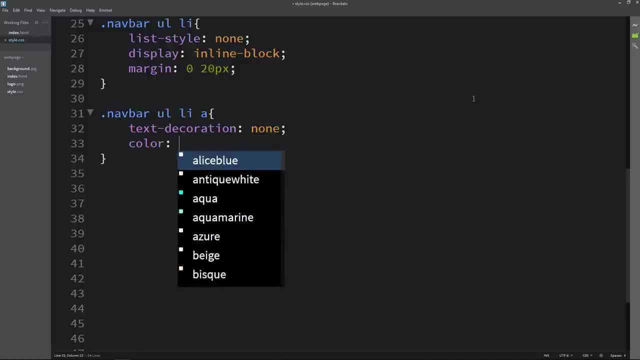 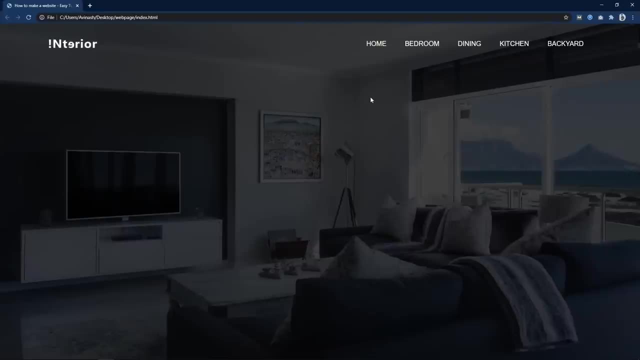 the anchor tag. here we will add text decoration will be none and color will be 0 and we will add text decoration will be none and we will add text decoration will be none and color white. then text transform uppercase. now it looks good. next we have to add the hover effect. 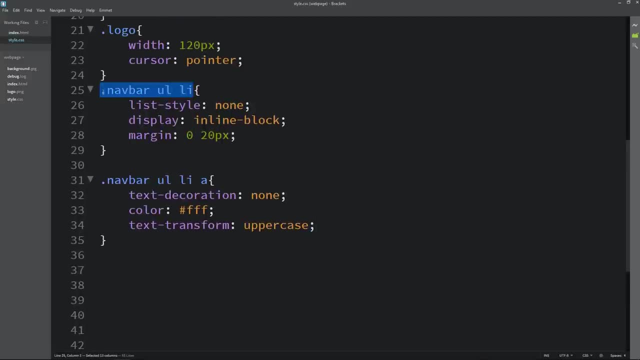 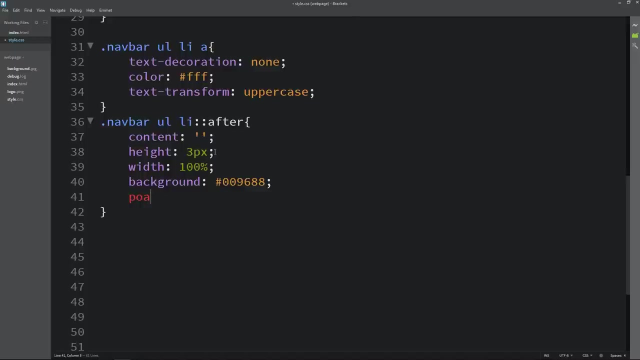 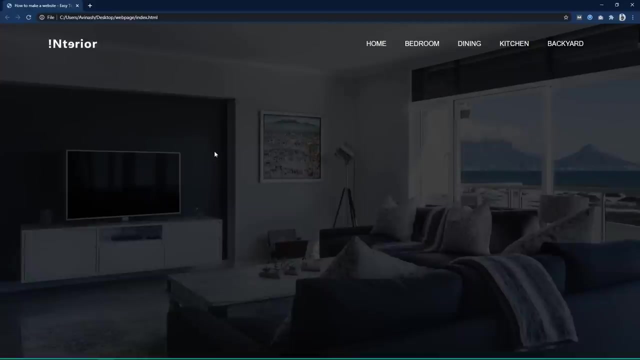 on these menu. for that, just come back and copy this one, then write after in this: after we will add content empty and height 3 pixel width 100 percent and background this color code. then position will be absolute left 0 and bottom 0. ok, it is coming at the bottom of the web page, so just come back and here in this li we will. 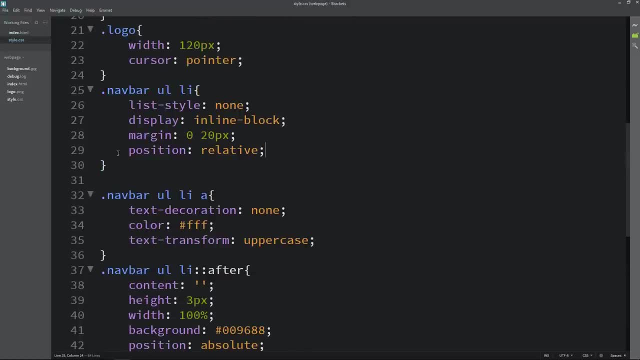 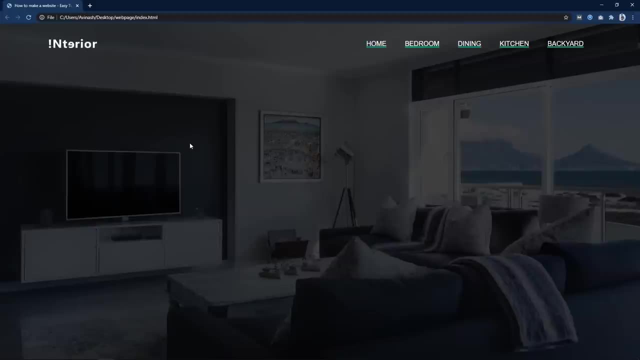 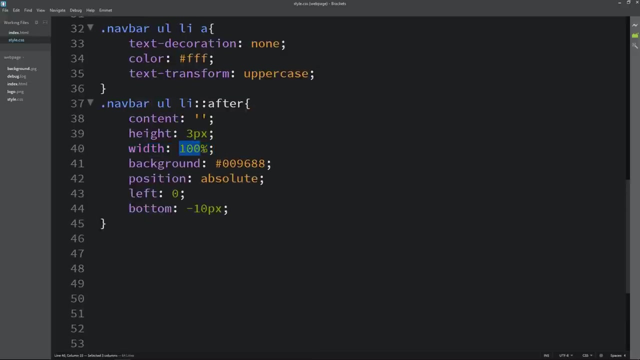 add position relative. after that you can see these line below the menu. next we have to add some space, so in the bottom we will add minus 10 pixel. now it looks good. next we have to hide all these line. so just come back and instead of 100 percent we will write width. 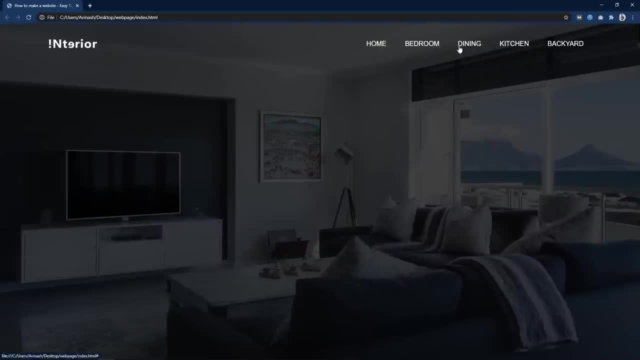